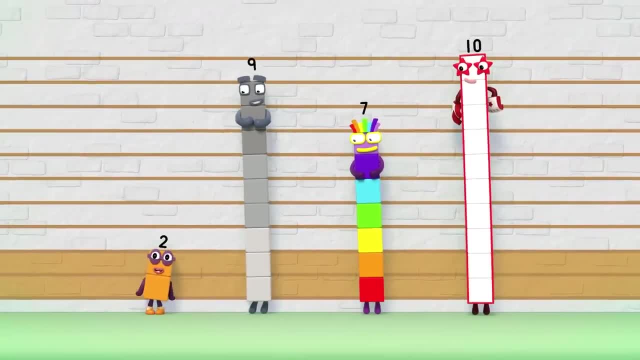 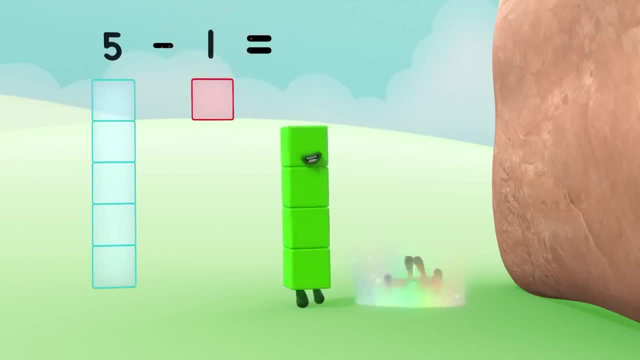 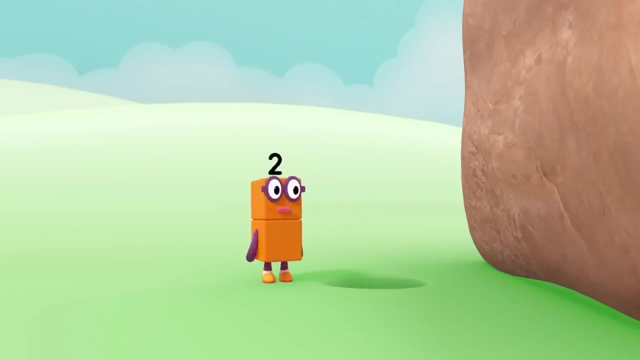 5.. So take off the difference and everyone will see what the difference is between you and me. 5 minus 1 equals 4.. 4 minus 1 equals 3.. 3, minus 1 equals 2.. 2 minus 1 equals 1.. 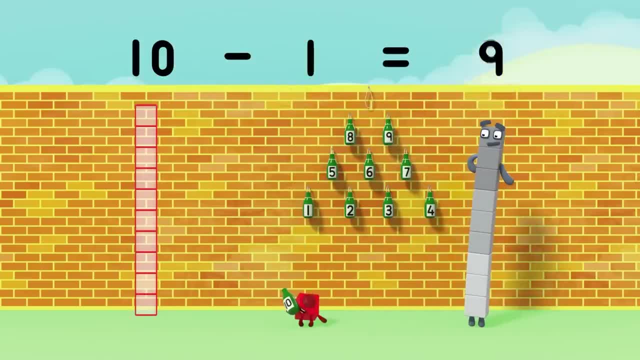 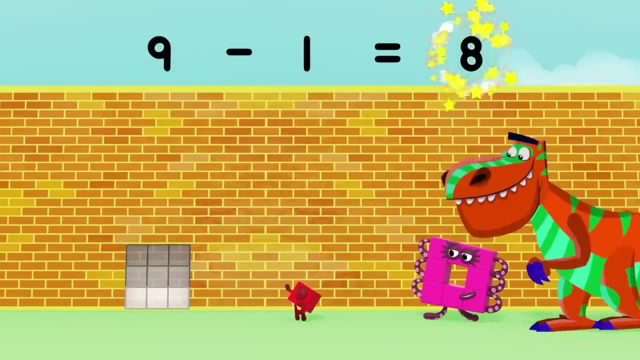 But one green bottle should accidentally fall, There'll be 1,, 2,, 3,, 4,, 5,, 6,, 7,, 8,, 9.. But if one green bottle becomes a dinosaur, there'll be one, two, three, four, five, six. 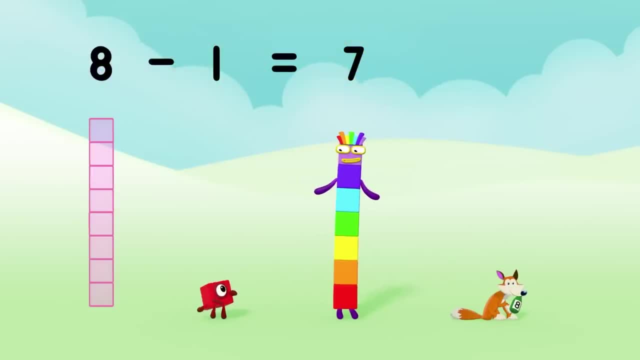 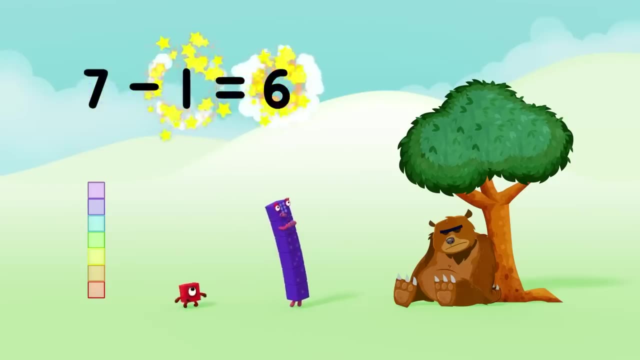 seven, eight. But if one green bottle is stolen by a fox, there'll be one, two, three, four, five, six, seven. But if one green bottle should wake a grizzly bear, what I mean? hug a teddy bear. 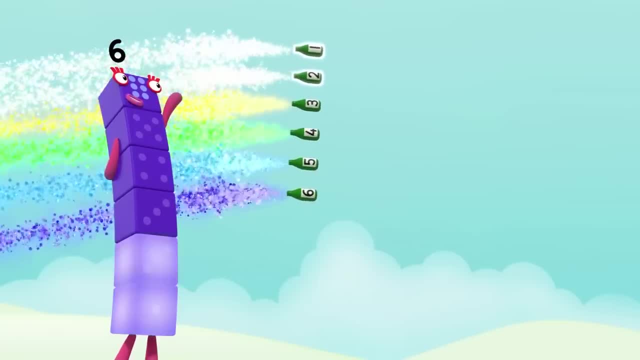 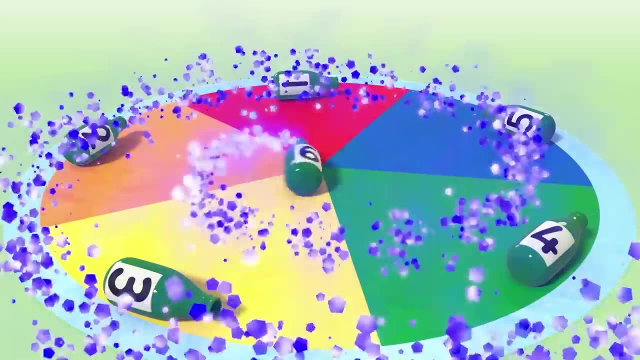 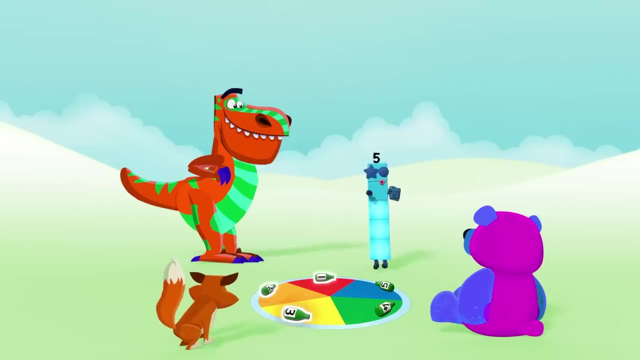 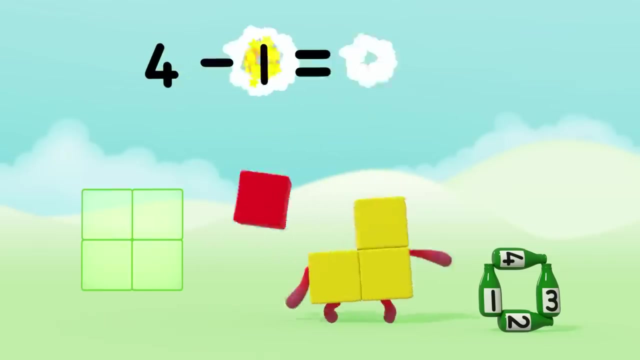 Phew, There'll be one, two, three, four, five, six. And if one green bottle spins around, whoa, you win. There'll be one, two, three, four, five. But if one green bottle should grow a daffodil, there'll be one, two, three, four. 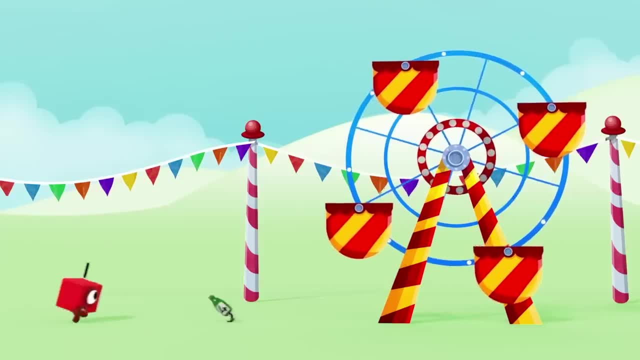 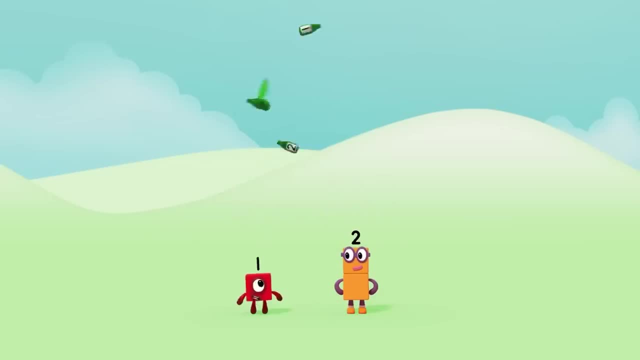 But if one green bottle should run to the bear, there'll be one, two, three, four, five, One, two, three. But if one green bottle Should pop its wings and fly, There'll be one, two, two green bottles Spinning in the sky. 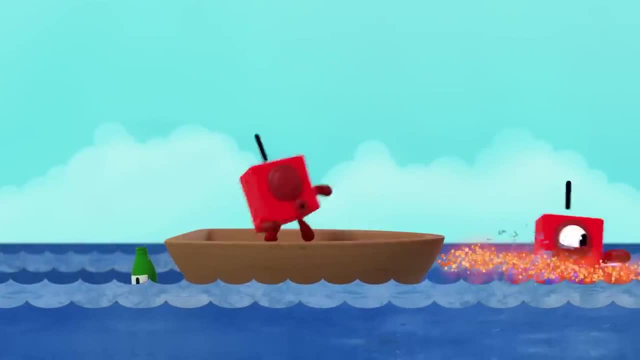 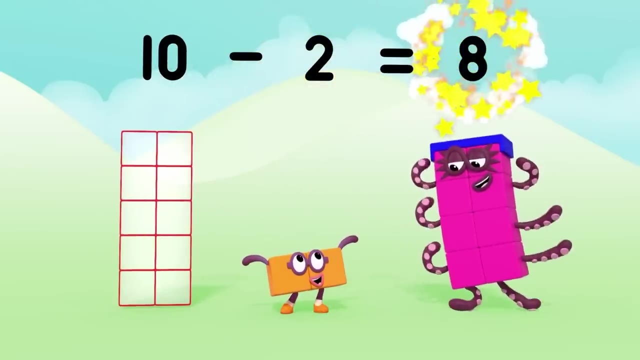 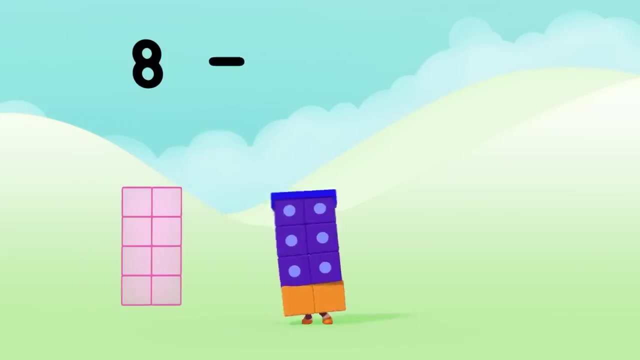 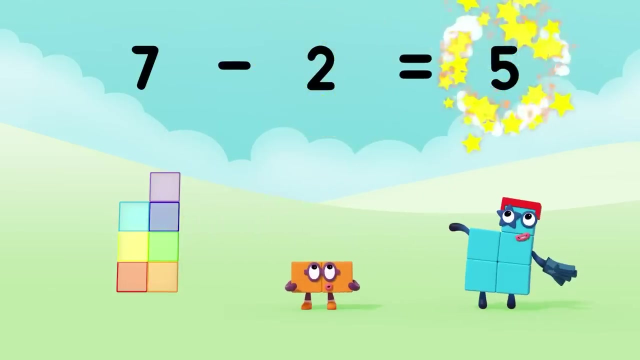 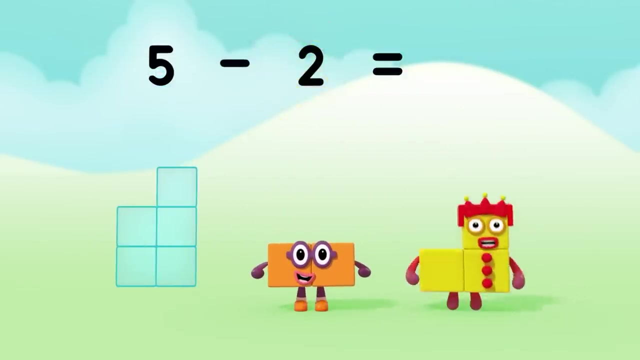 But if one green bottle Should learn to water sea, There'll be one one green bottle Floating out to sea. Ten minus two Equals eight. Nine minus two Equals seven. Eight minus two Equals six. Seven minus two Equals five. Six minus two Equals four. Five minus two Equals three. 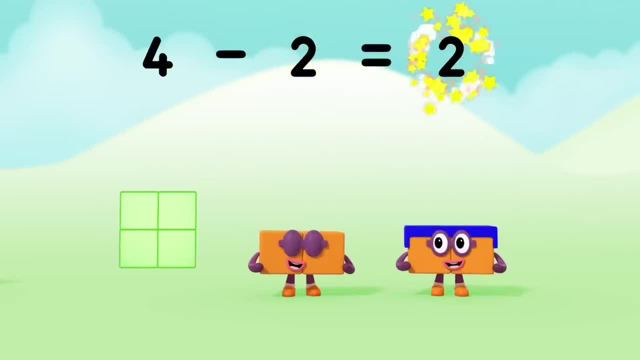 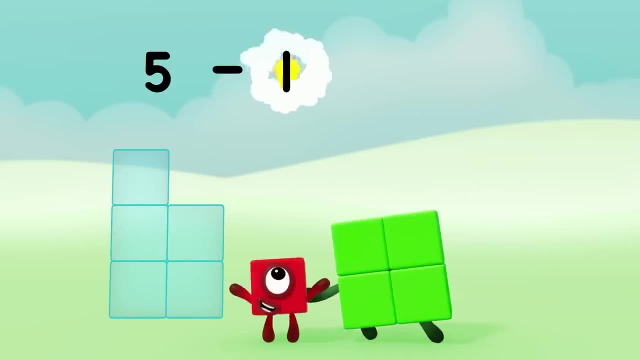 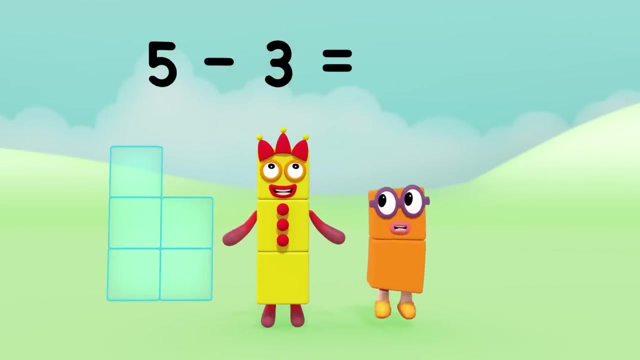 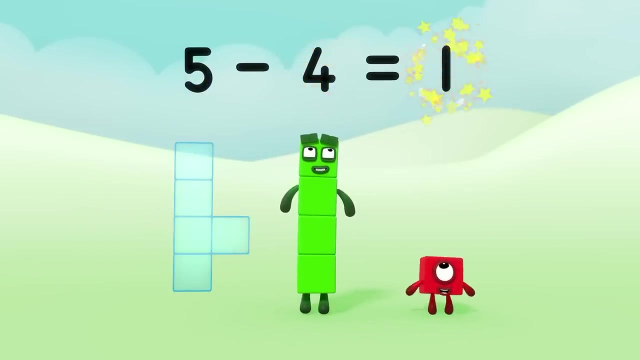 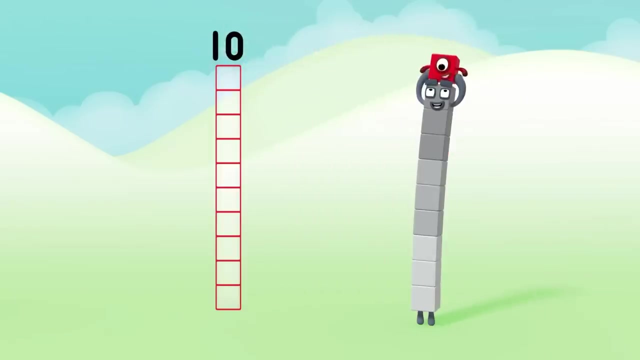 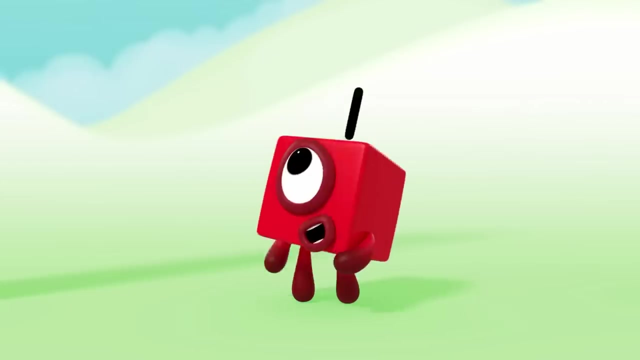 Four minus two Equals two. Three minus two Equals one. Five minus one Equals four. Five minus three Equals two. Five minus four Equals nine. Five minus four Equals one. Five minus two Equals three. Ten minus one Equals nine. Ahhh, You're amazing, One bigger. You're one bigger. 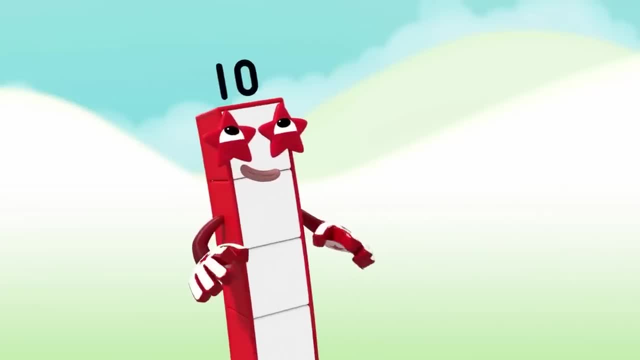 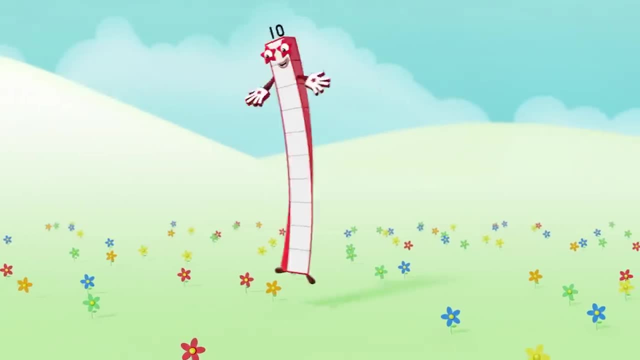 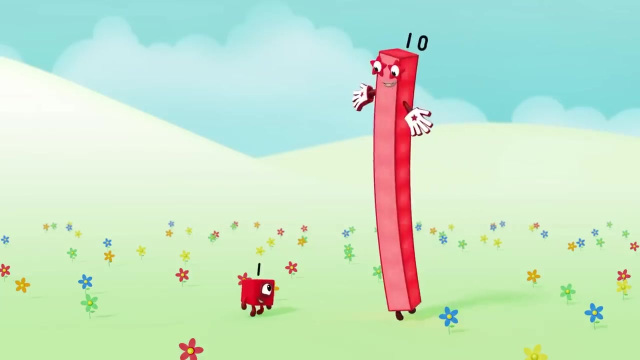 Why do you have a one on top? One bigger, One bigger. If you're wondering why there's a one on top, You'll know the answer when you realise: I'm one big block, I'm one big, perfect ten. I'm a ten block, I'm a ten block. 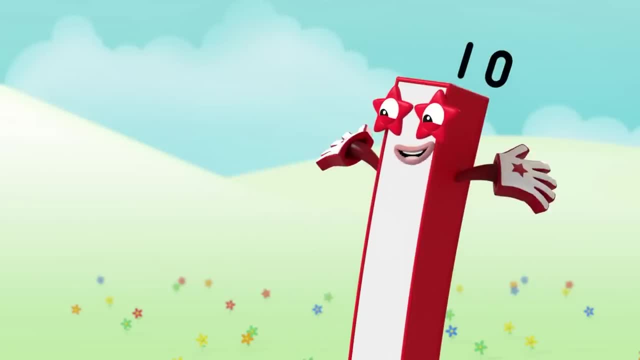 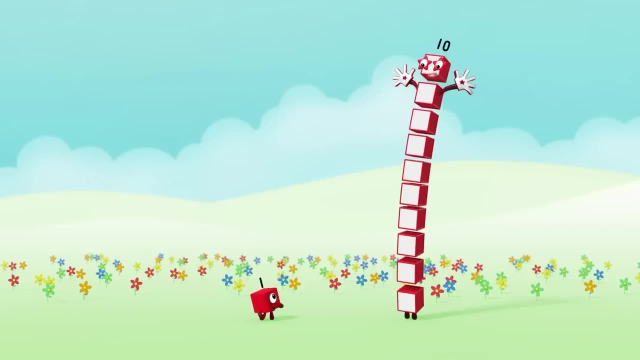 You might think we're different. think again. We're more alike than you suppose. You're one one and I'm ten ones, Which means I'm one ten One, two, three, four, five, six, seven, eight, nine ten. Two is made of two blocks. 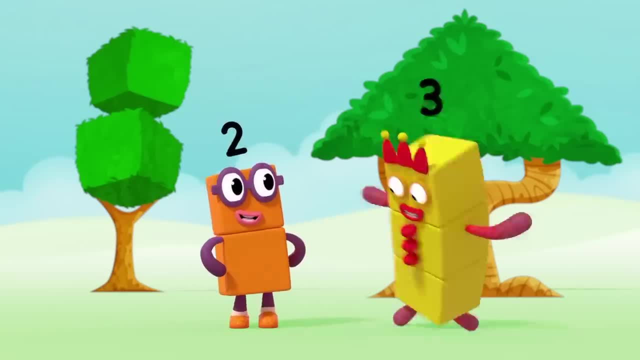 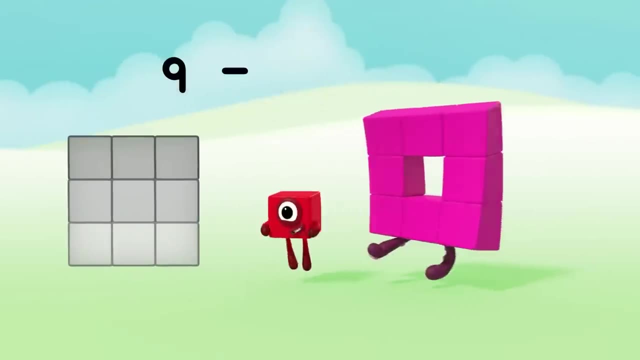 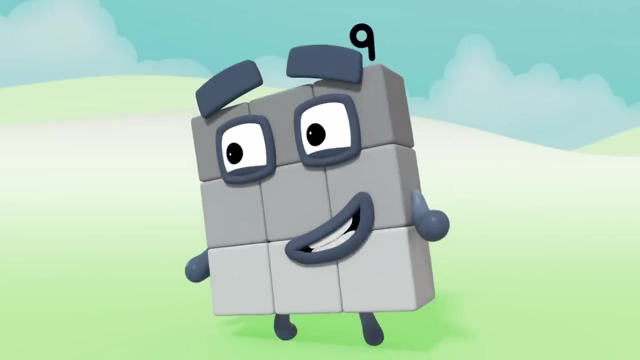 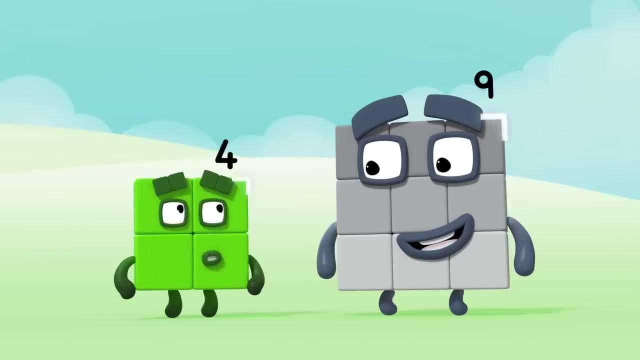 I'll always be your friend. Three will entertain you On what you can depend. Minus one Equals eight A square, Yes, One, two, three, four, Four sides Like me. One, two, three, four, Four corners Like me. Yes, I'm a square. 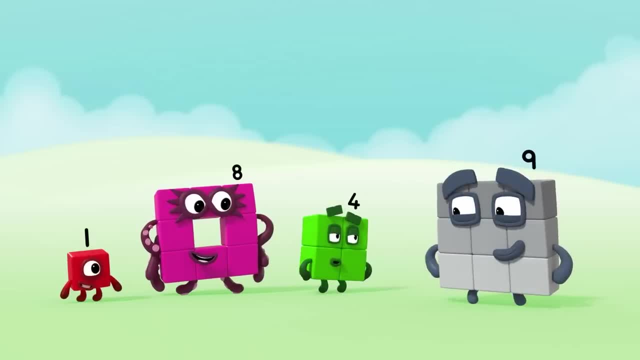 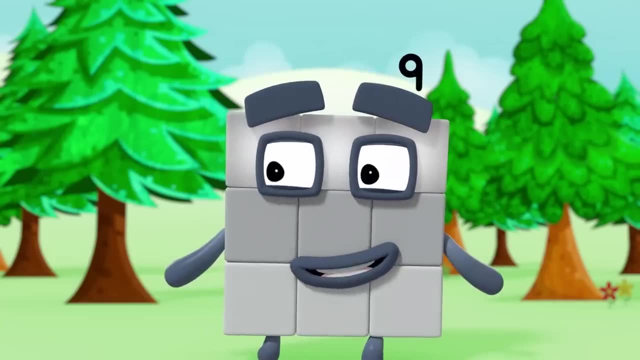 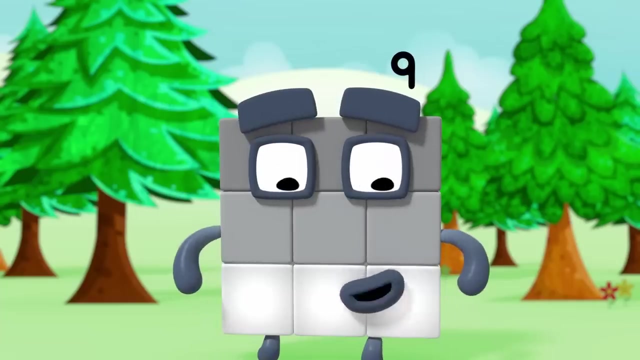 Like you. So why do you have a number nine on top silly? I'll show you One, two, three, Three blocks in my first row. One, two, three, Three blocks in my second. One, two, three, Three blocks in my third row. 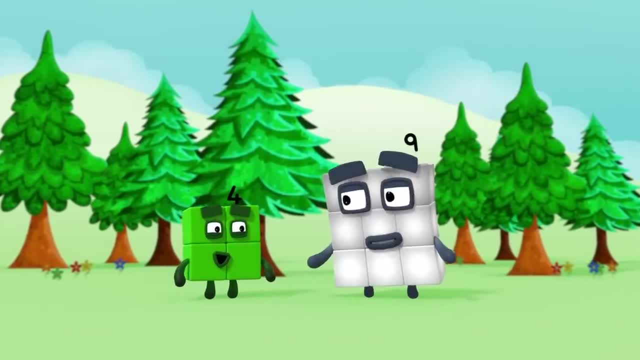 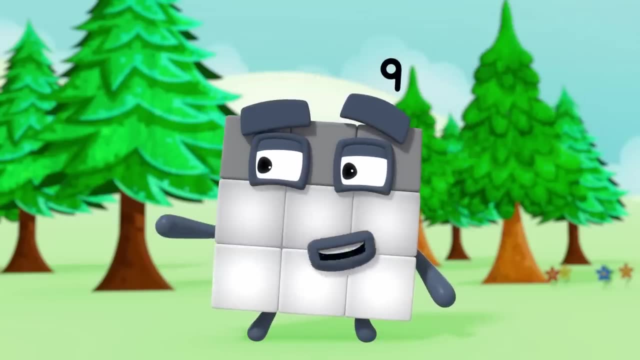 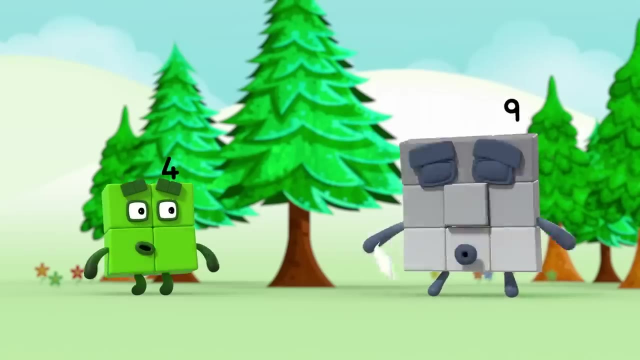 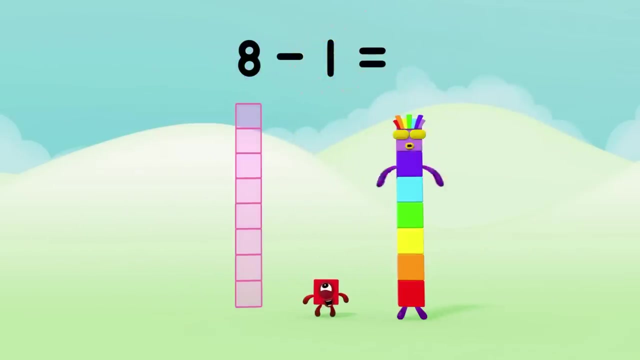 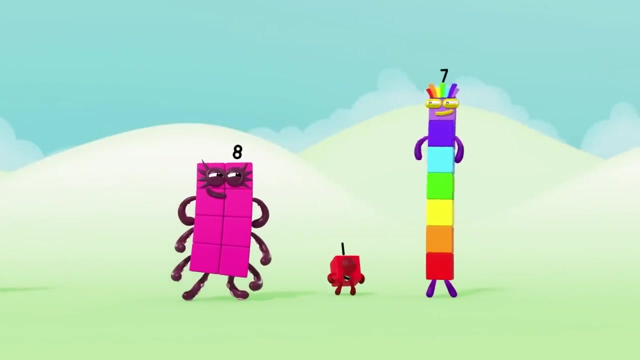 Three blocks in my second row, Three rows of three. Three rows combine, As you can see. Three rows of three make nine. One, two, three, four, five, six, seven, eight, nine, I'm fine. Eight Minus one Equals seven. Hey, Wow, Told you that was a lucky hop. 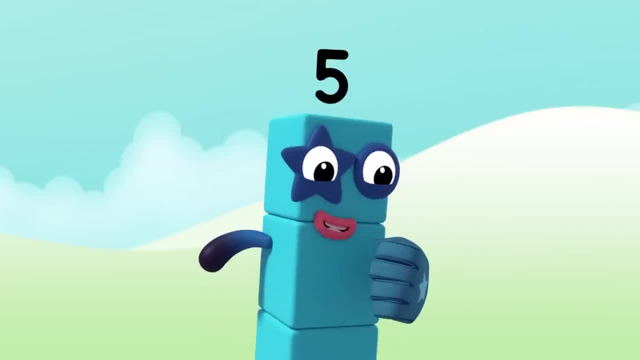 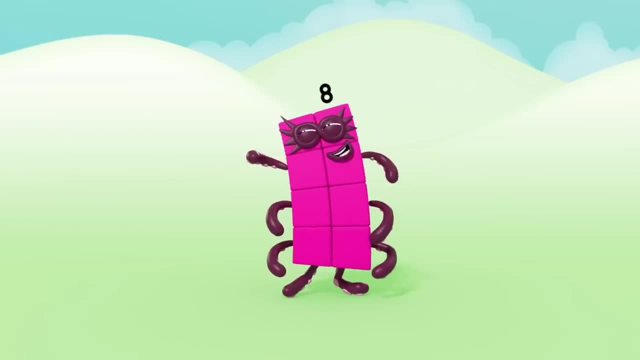 Hello, Hey there, You're very good at waving. That's not all I can do. Who are you? I'm Eight, but you can call me Octoblock One, two, three, four, five, six, seven, eight. 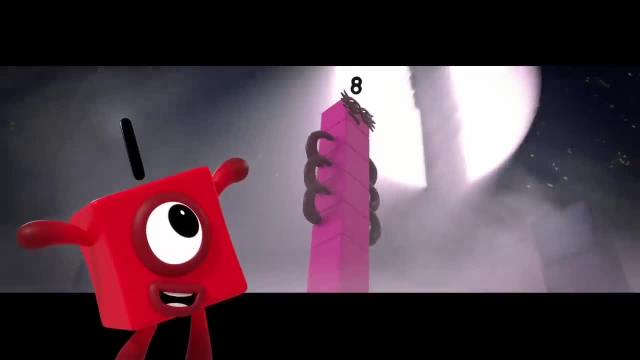 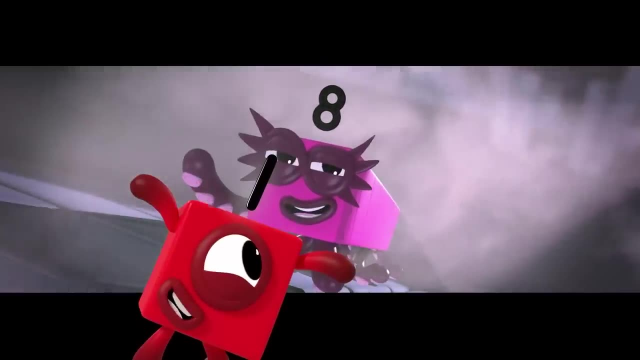 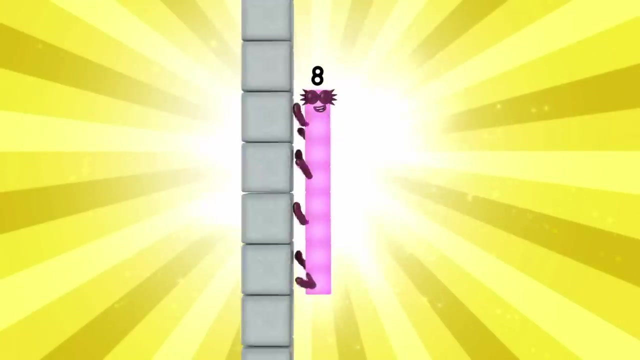 He can stand really tall. He can climb up the wall. He is Octoblock, Octoblock, Octoblock. climb One, two, three, four, five, six, seven, eight climb. He can stand like a pillar or make himself wider. 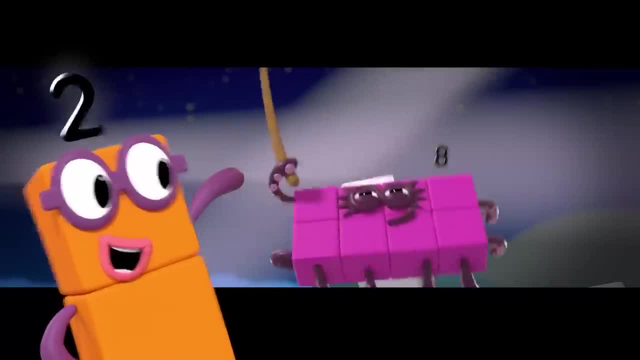 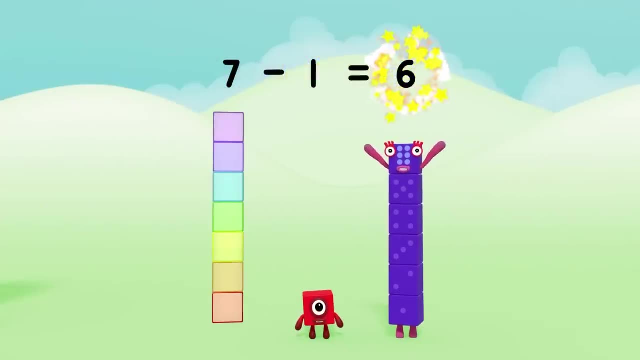 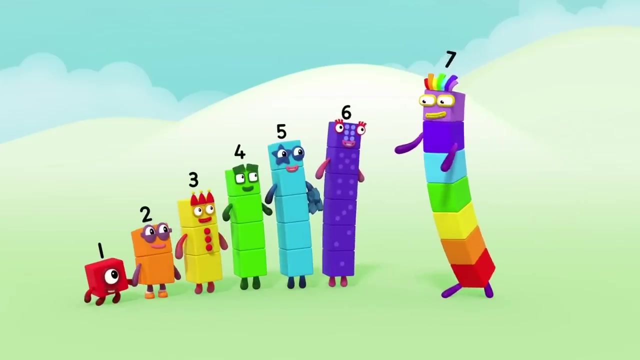 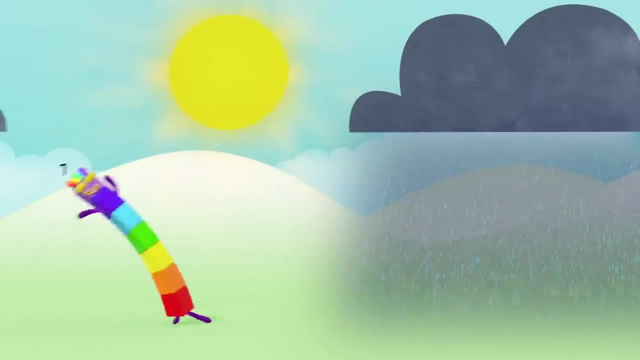 and crawl like a creepy rectangular spider. He is Spider-Blob. Oh, hang on. Octoblock Seven minus one equals six. All you lovely blocks are my friends. I'm the luckiest number block in the world. I'm lucky number seven. 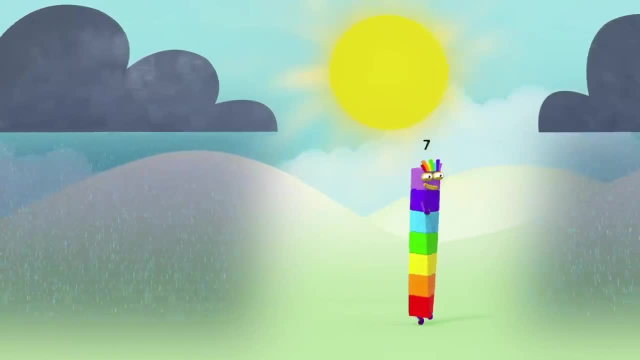 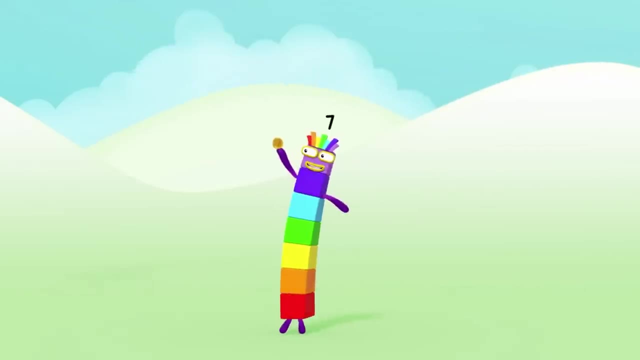 I'm in a happy place, The sun is always shining and there's always a smile upon my face. I see a penny and I'm here to pick it up, And all day long I have good luck. I'm lucky number seven. 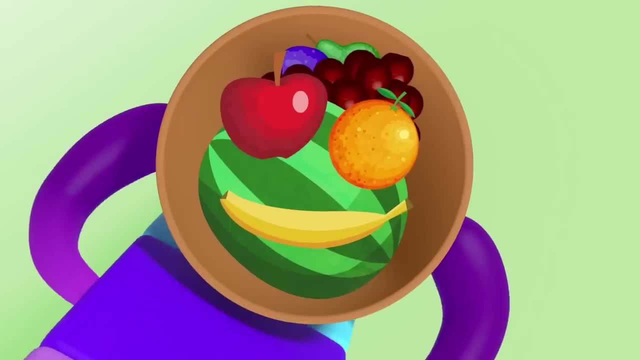 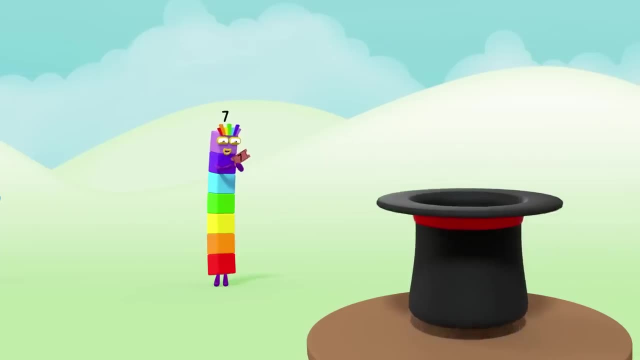 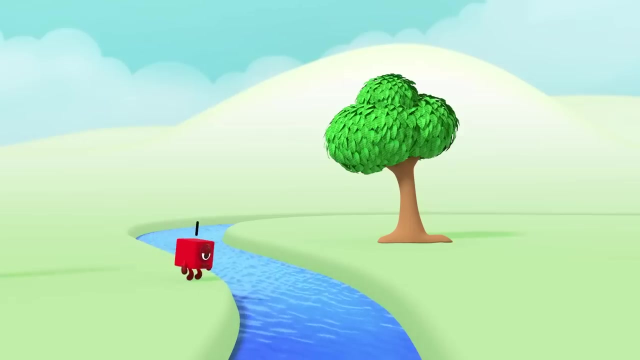 and everything is falling into place. I'm lucky number seven and, as you might have guessed, I always win the raffle With seven on your side. you're seven blessed In a pickle. you're in luck. I'll help you out when you get stuck. 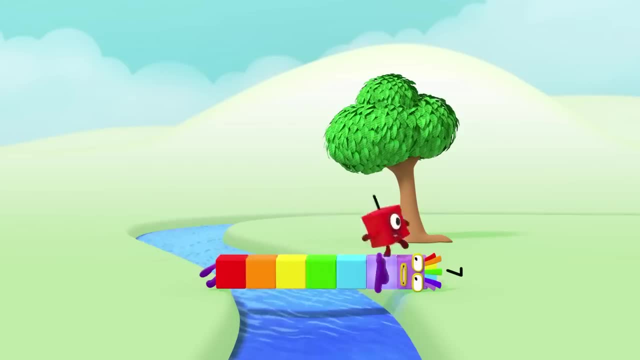 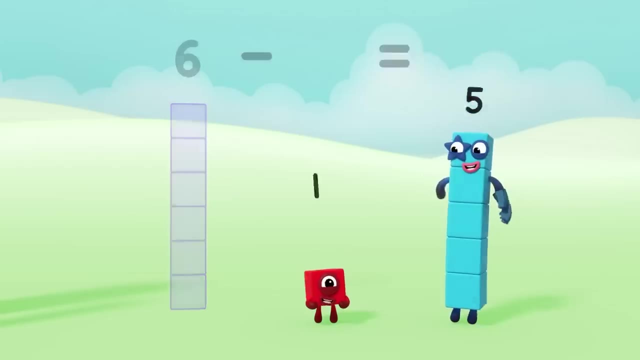 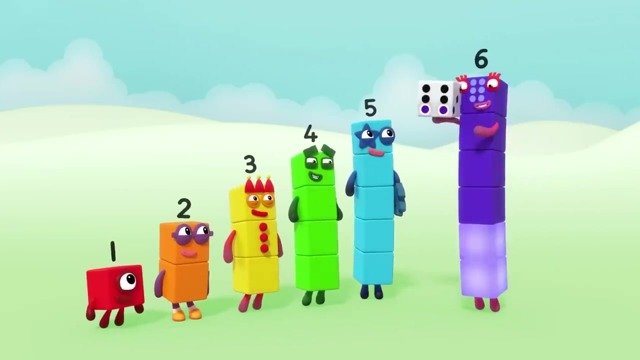 And if you stick with seven, everything will work out for the best. Six minus one equals five, Six minus one equals five. Six minus one equals five. Oh hey, One, two, three, four, five, six. One, two, three, four, five, six. 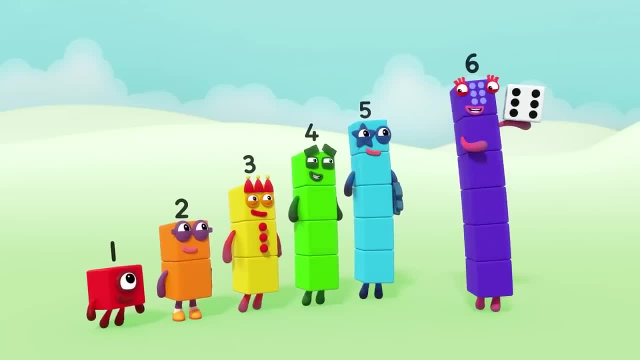 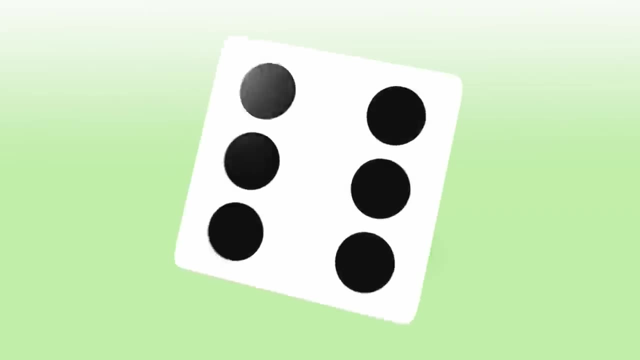 One, two, three, four, five, six, Six spots, just like me. What is it? This little block is full of tricks. It's got six faces, one to six. It's called a die. it's called a dice. 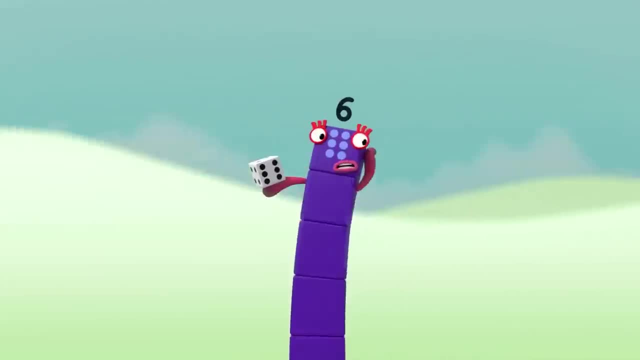 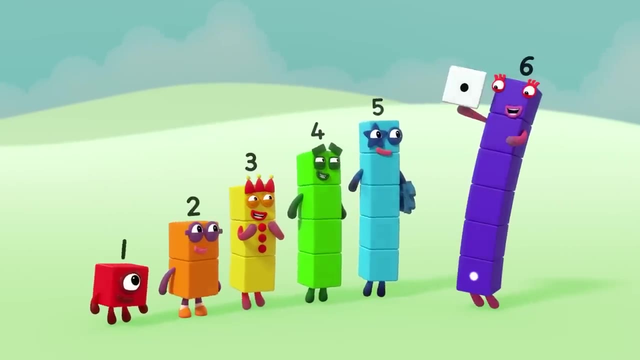 It's called a die. it's called a dice Or die. both names are nice. What's it for? Let me explain. Want to know more? Let's play a game, And this game goes like this: When you see a number, make the shape. 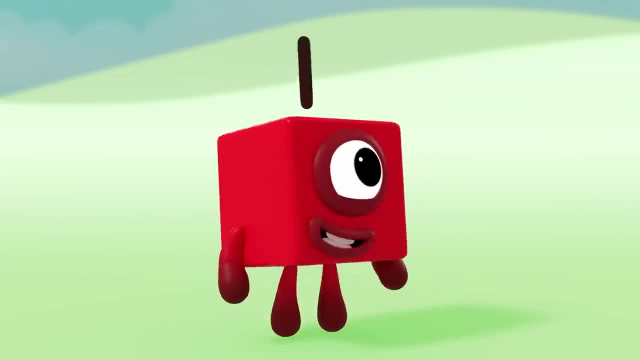 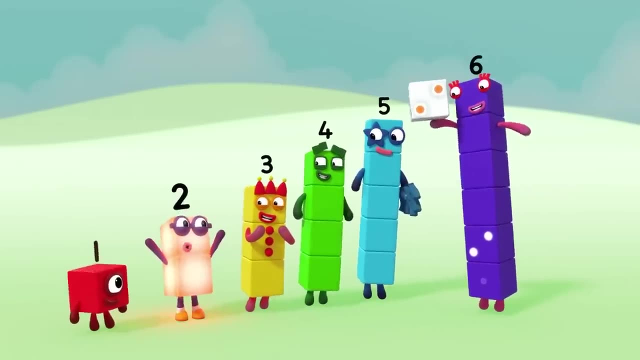 One. One spot on the dice. Make the shape One, One, two, two spots on the dice. One, two, two spots on the dice One, two, two spots on the dice. Make the shape Two, One, two, three. 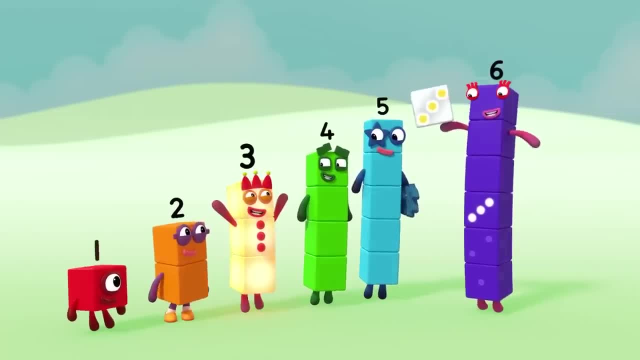 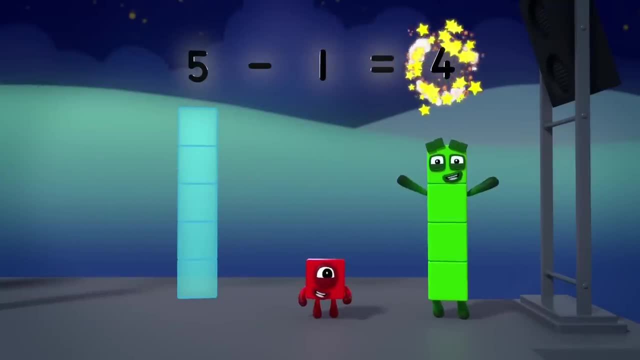 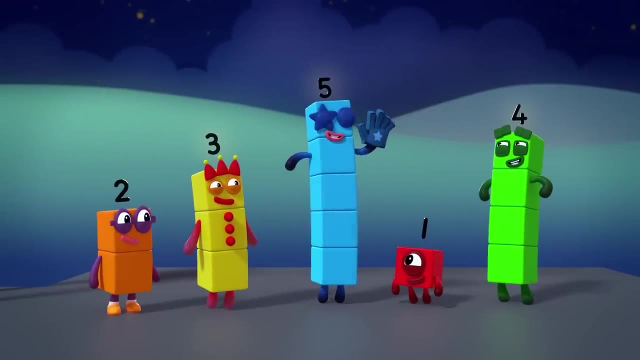 One, two, three. One, two, three, Three spots on the dice: Five minus one. Five minus one Equals four, Equals four. And who are you? I'm Five, And you can count on me to get this party started. 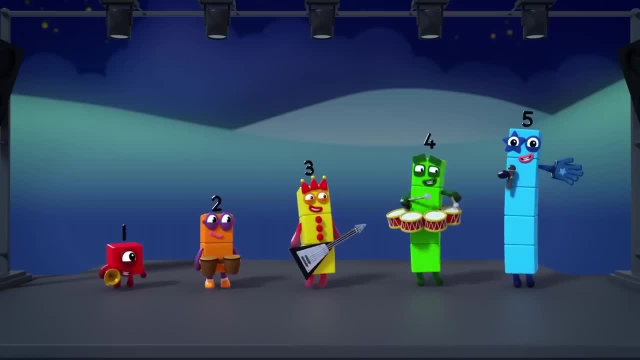 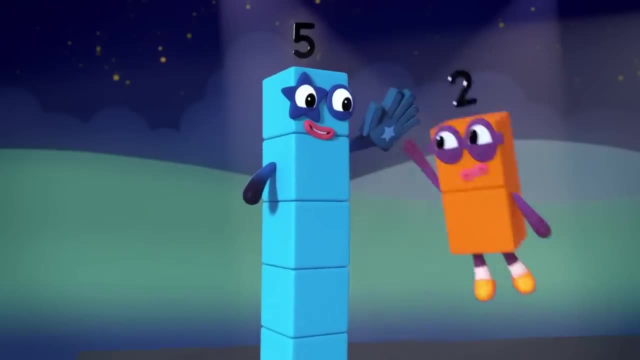 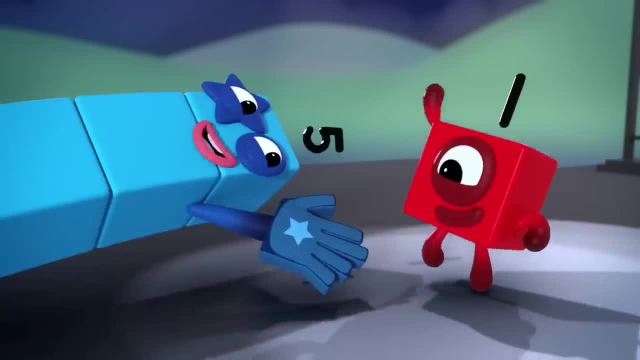 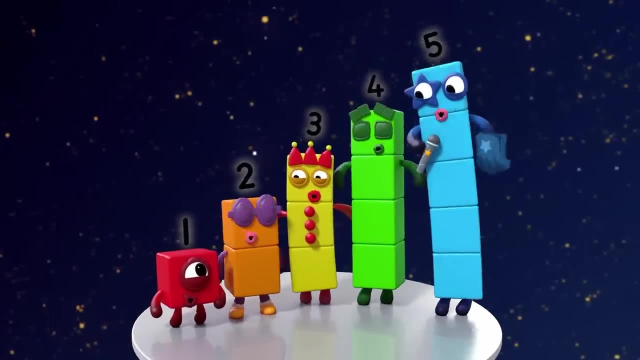 High five To the side, Up above, Down low, Too slow. High five. Ooh, I feel so alive. You know that you've arrived when you're with number five. Five points on a shooting star: One, two, three, four, five. 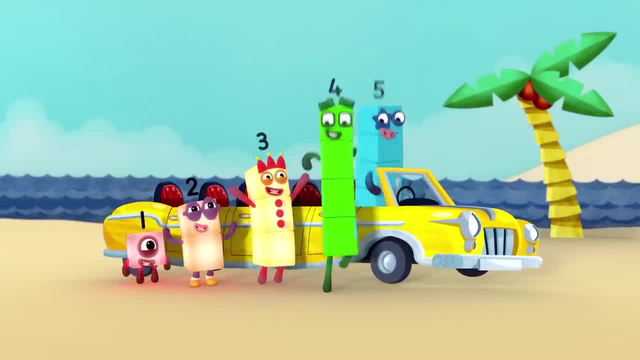 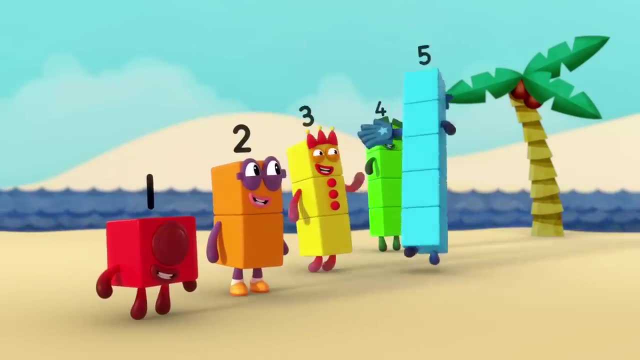 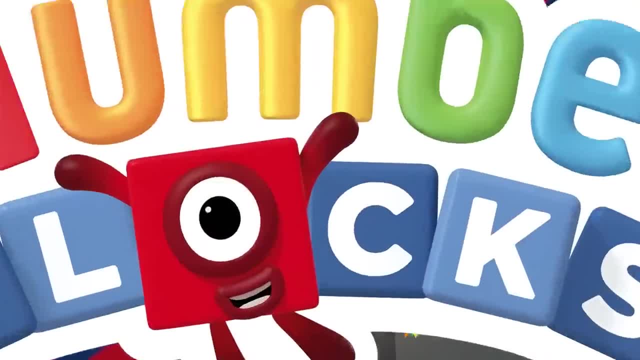 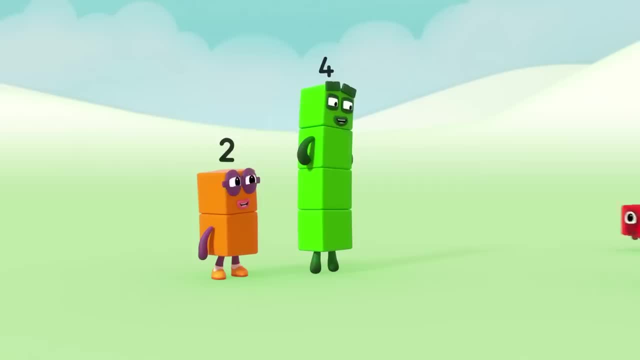 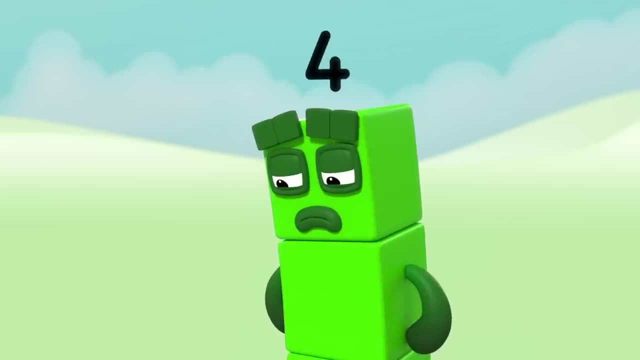 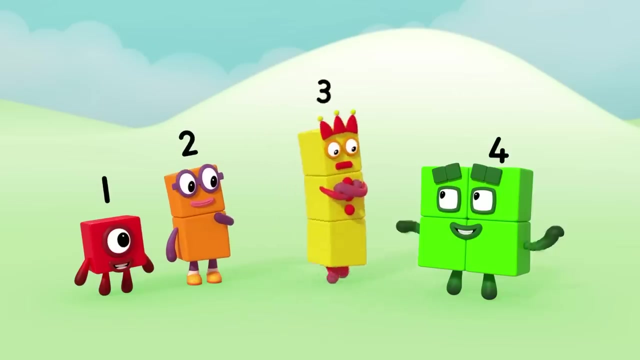 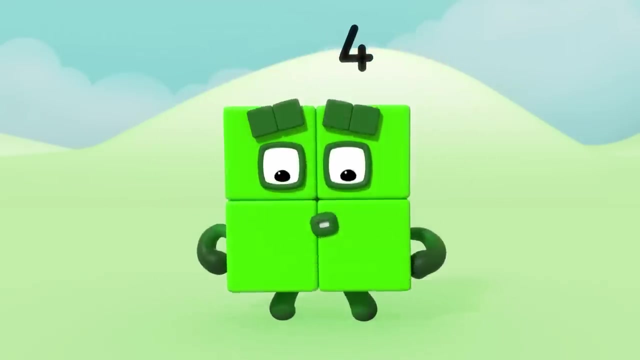 To the side, Up above, Down low, Too slow. Four minus one equals three. This won't do. I'm three. I want to be the biggest. I can be shorter, That's much better. Ooh yeah, I am square. 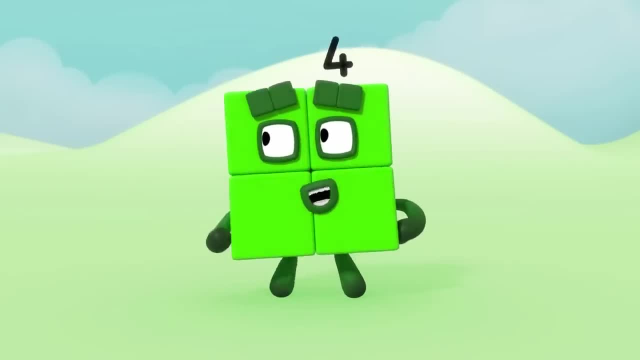 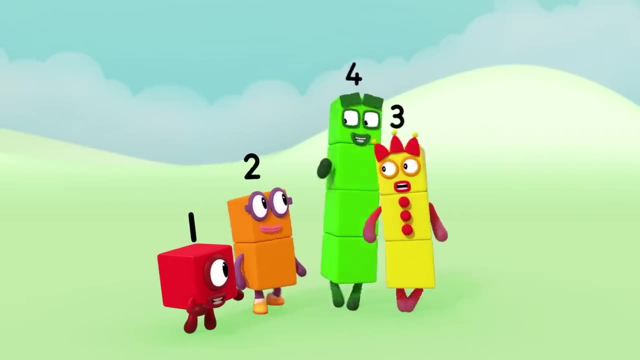 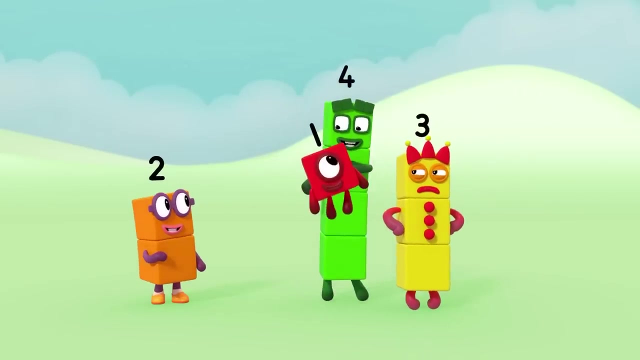 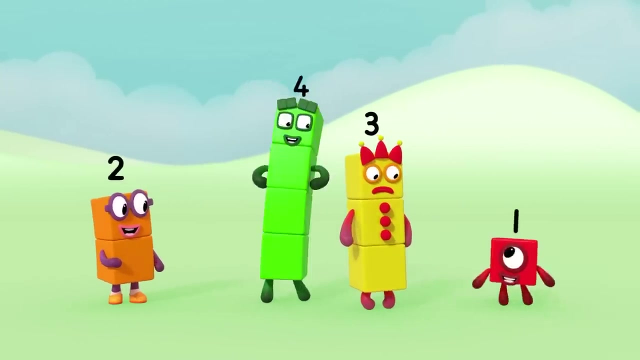 What's so special about being square? I'm so glad you asked. I'm four. Have you met me before? I'm one more than three. That's plain to see. Three plus one equals me. I'm four. One, two, three, four. 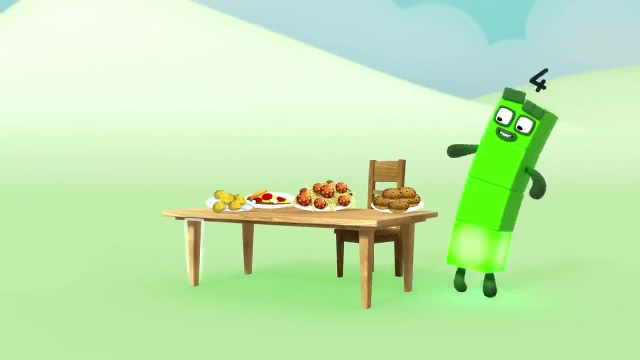 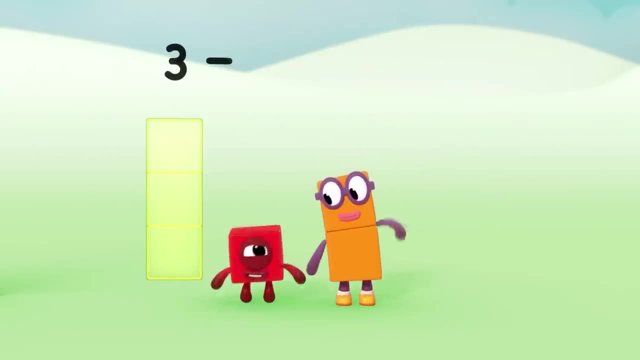 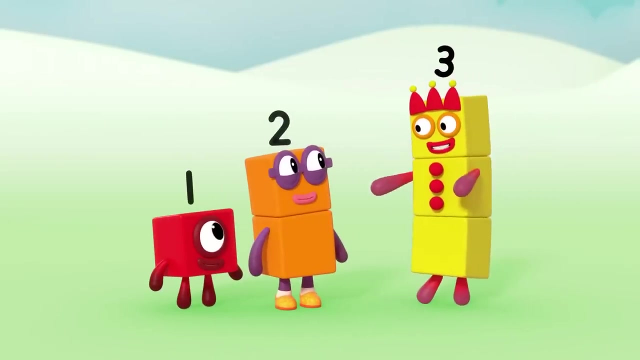 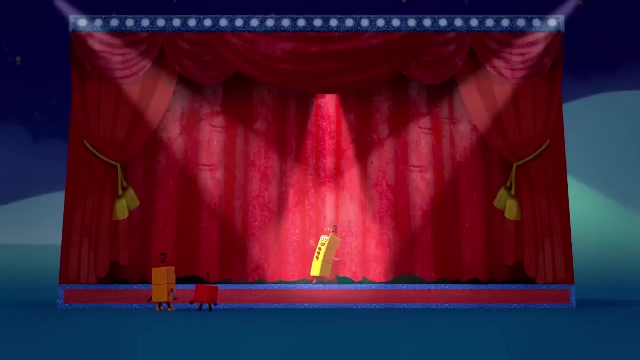 Four legs on a table: One, two, three, four. Four legs make the table more stable. Three minus one equals two. My audience, That's better Ready. Three, One, two, three. Everybody, look at me, I'm here to entertain you. 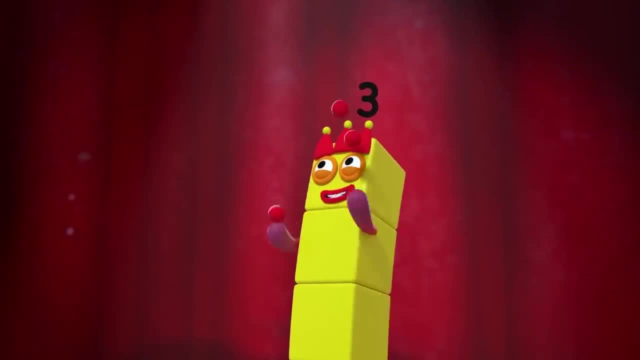 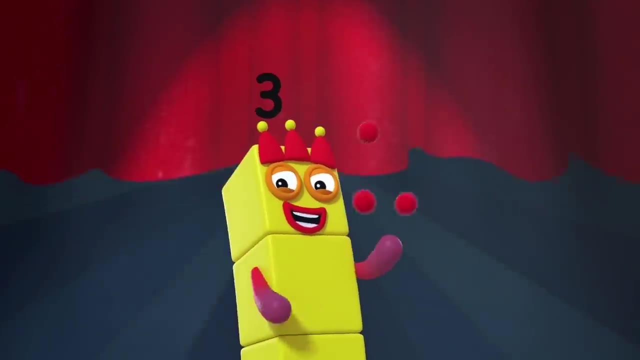 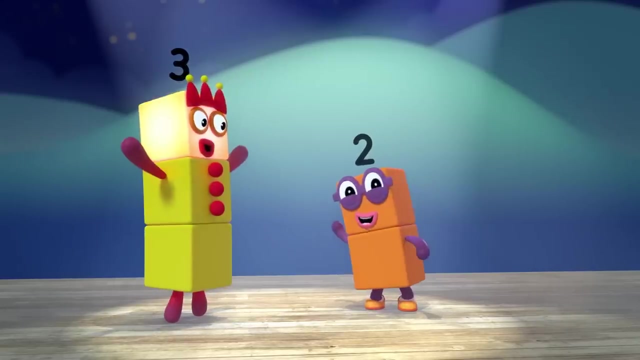 with this funky melody. I'll juggle three balls in the air and everyone will cheer. Everything's gonna be all right Now. number three is here. I'm in tic-tac-toe, I'm in ready. steady go. You're gonna have to count to three. 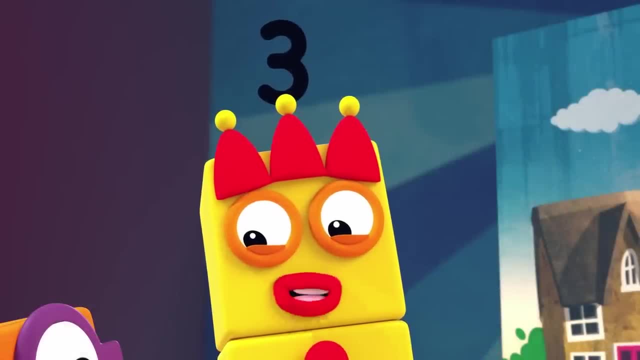 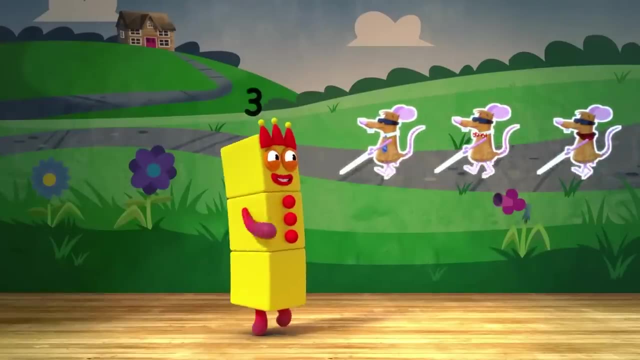 to get three in a row, You'll find me hiding everywhere you look in a fairy tale or a picture book. One, two, three, Can't you see I'm in? three blind mice, Three wishes. would be nice. You should try and try and try again. 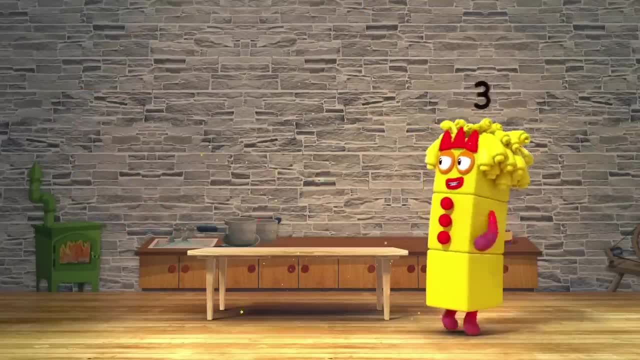 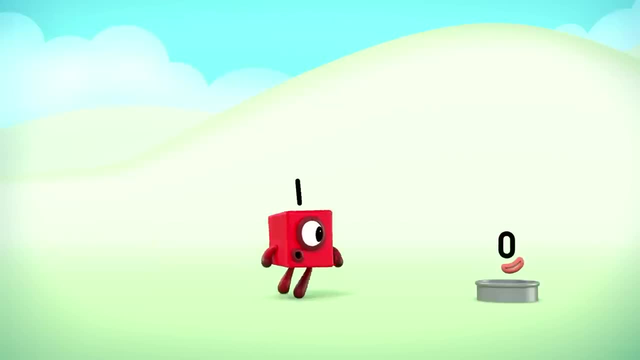 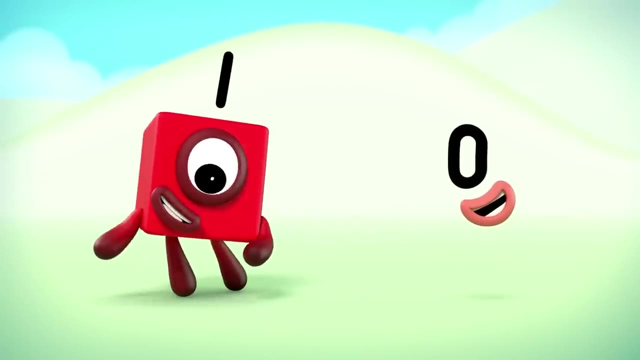 That's my advice. Goldilocks came across three bears. One minus one equals zero. Who are you? I am zero. the hero, One less than one. Where are your blocks? I haven't got any silly. Zero blocks. 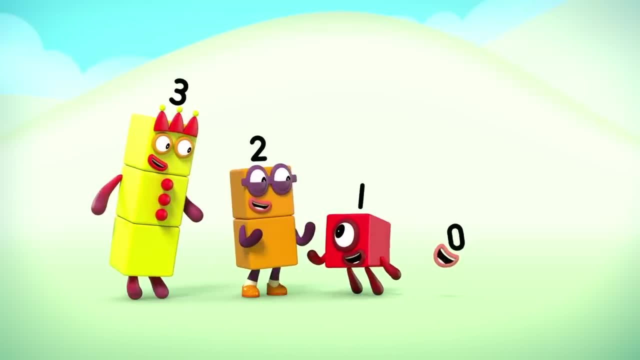 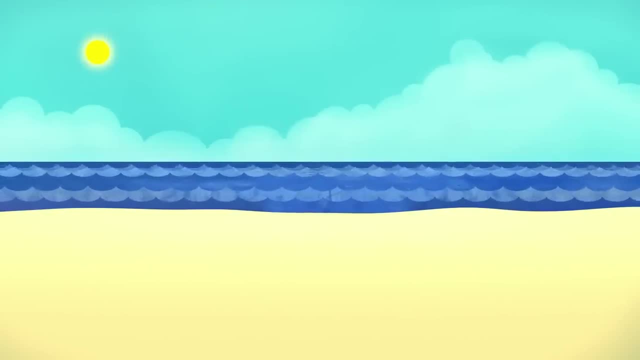 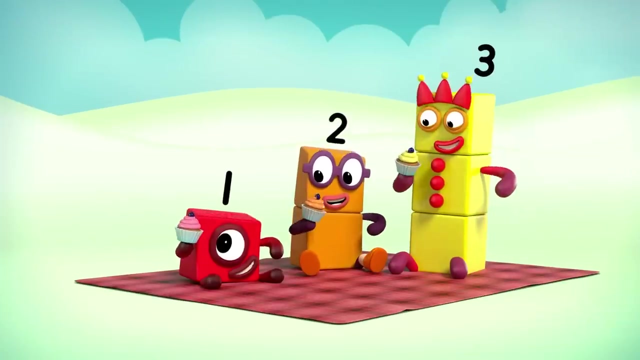 Wait, is that no music? I hear, Follow me. When there are no boats anchored in the bay, you've got zero. When all the birds have hopped and flown away, you've got zero When you've eaten all the cupcakes.